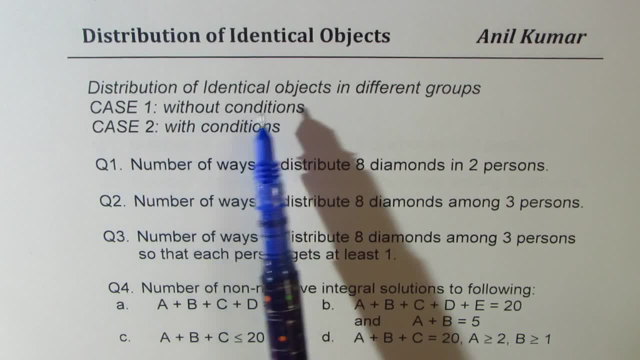 groups. We'll have two cases, one without conditions and the other with conditions. right Based on these cases, here are four questions. Question number one: number of ways to distribute eight diamonds in two persons. Question two: number of ways to distribute. 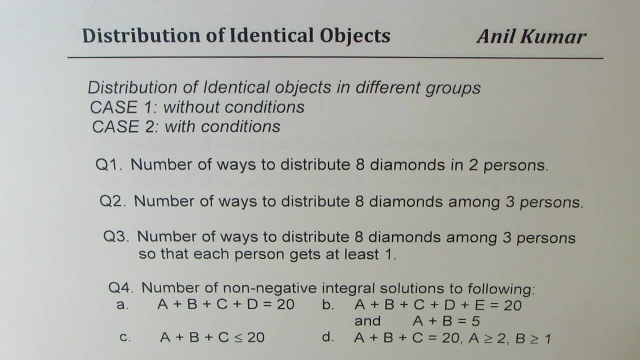 eight diamonds among three persons. Three: number of ways to distribute eight diamonds among three persons so that each person gets at least one. So that is kind of a condition, So that belongs to me And I'm going to talk about distribution of identical objects. 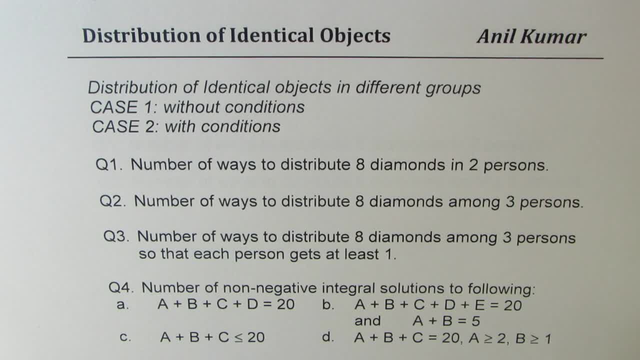 to case two, Question number four: Number of non-negative integral solutions to following equations. Now we have four different types of equations. It's a good variety to begin with. We'll take up more equations in the next part of the video. So let's begin by understanding. 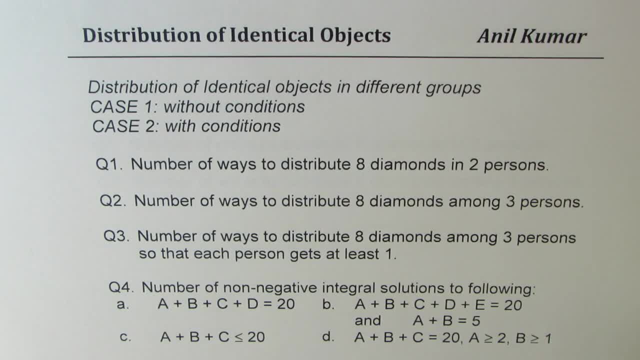 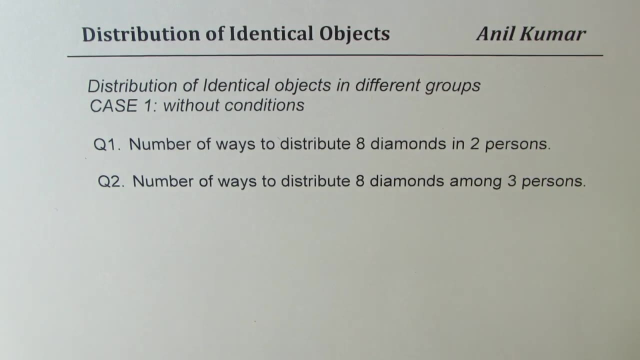 the concept and then we'll apply those tricks to solve these questions very fast, right? That's the whole idea: To save some time, especially for multiple choice questions, correct? So let's begin with case one, without condition. Now, here we have. we need to find number of ways to. 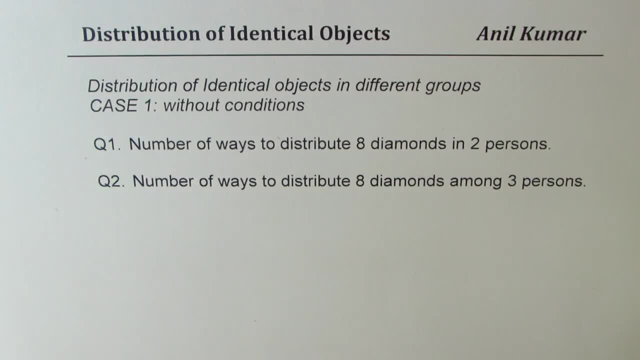 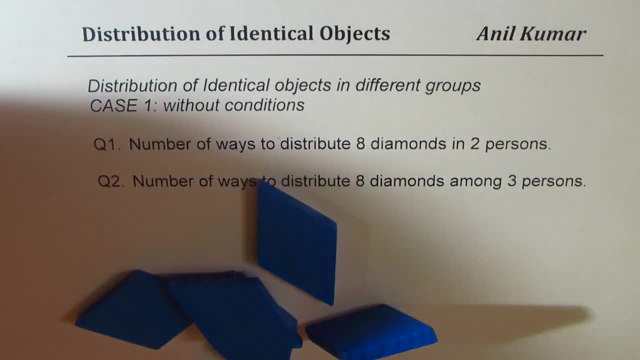 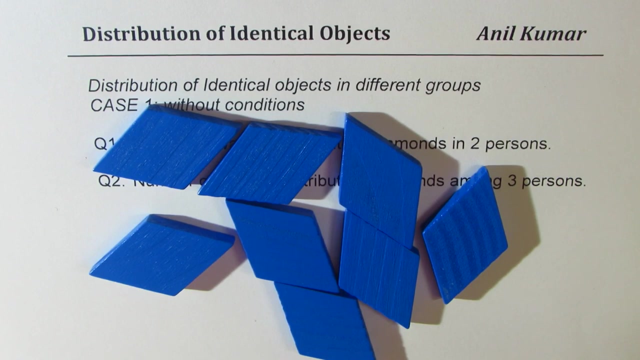 distribute eight diamonds in eight persons. Now, when we have to distribute, why not Distribute diamonds, correct? So let's say these are the eight diamonds for us, right? So these are eight diamonds and we need to distribute them to two different persons, correct? Now in 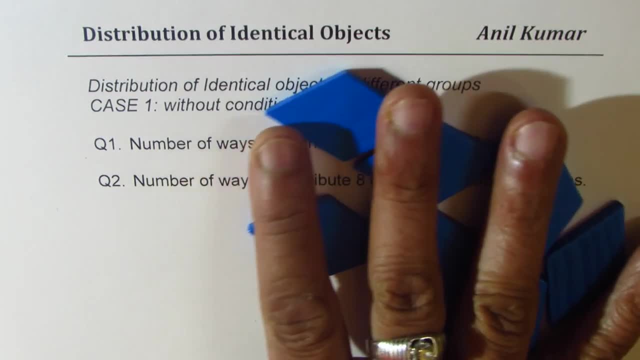 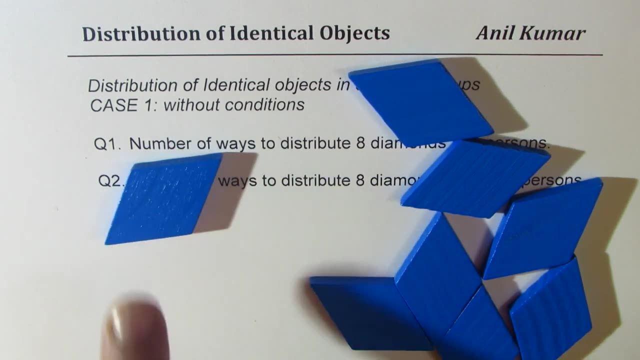 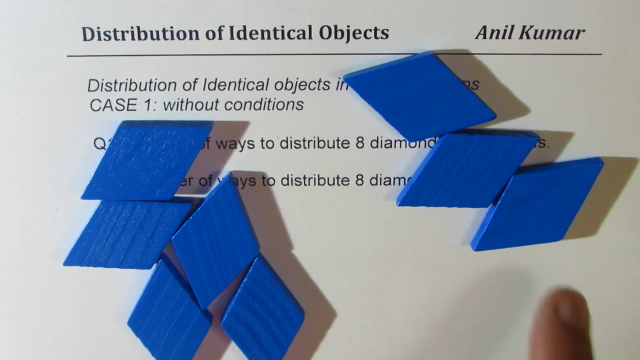 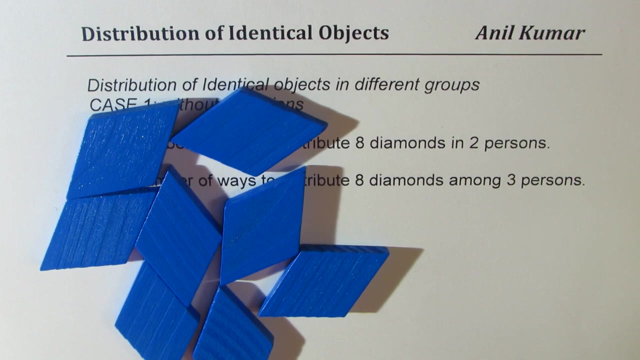 that case, condition could be that one person gets nothing, the other one get all eight, right, That could be the case, since there is no condition. Or we could have combination: one, seven, two, six, three, five. So we can get four, four, five, three, six, two, seven, one or all eight to the other side, right? So 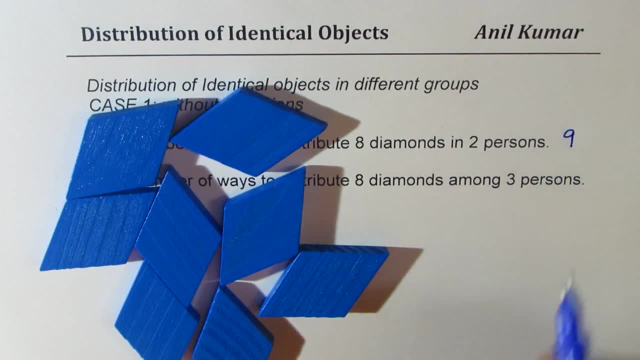 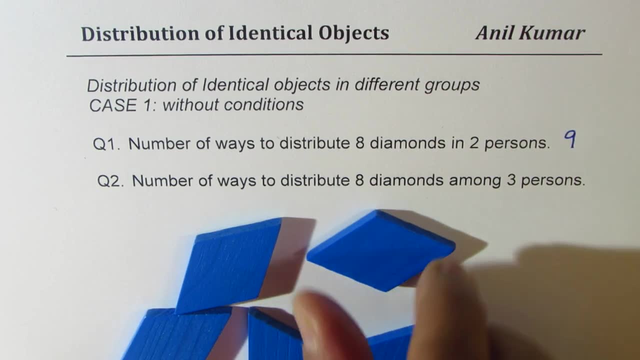 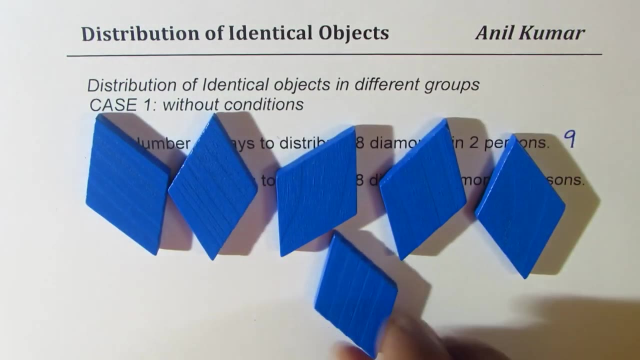 that gives you nine particular ways of doing it. Is that clear, right? So that gives you nine particular ways. Now, that was simple. The numbers are very small, so we could easily figure it out. Now, how do we apply what we've learned in permutation and combination to get a fast? 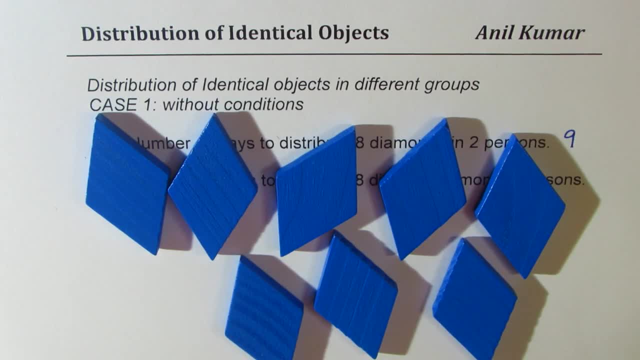 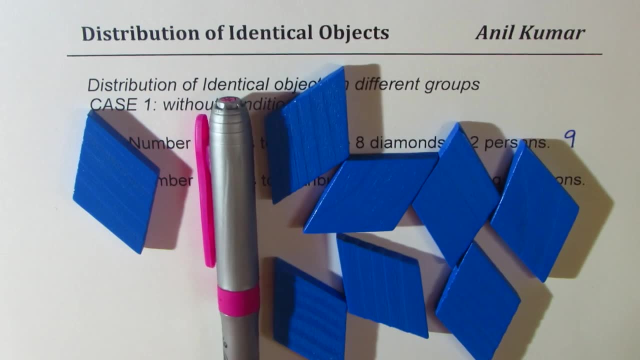 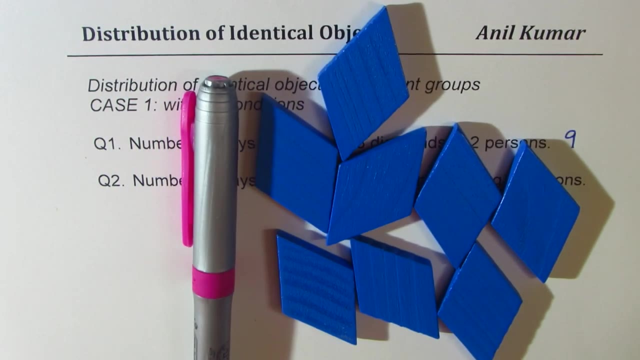 answer to this question. well, what we could do here is that we could use a line as a separator right, like this. so this divides into two groups. do you see that correct? so, so we could divide like this. so this is like one person getting all eight, the other getting nothing, and then, in this position, what we get is one. 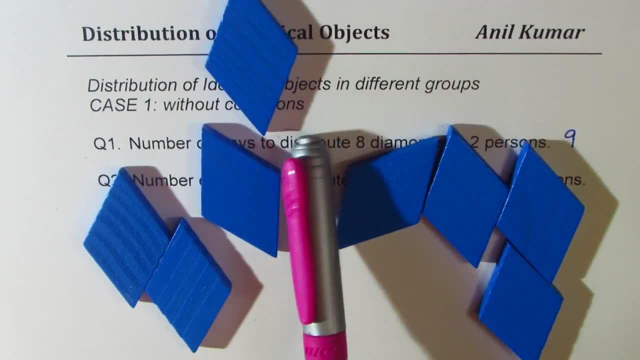 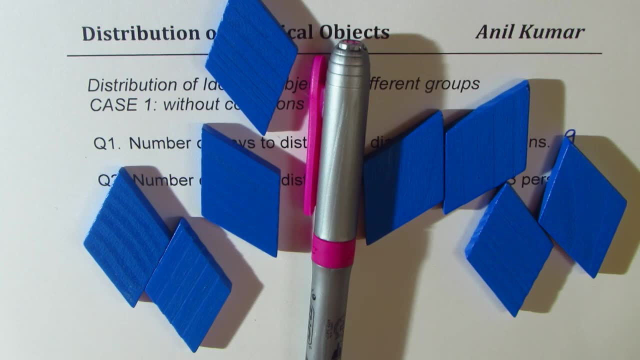 and seven, and then this is two and six, three or four, four or something like this. do you see that? so we have a position kind of like this, where we introduced another item which is different from those like items, correct? so let me show that different item using this particular block. okay, so what do we? 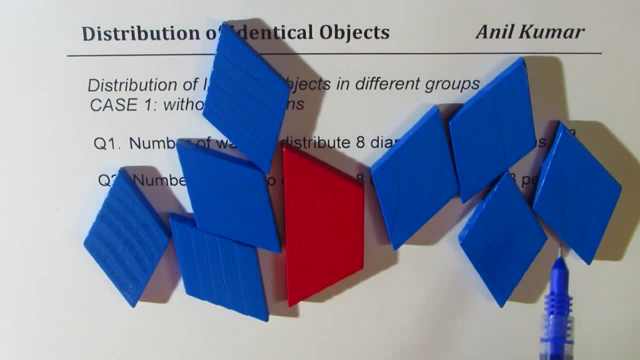 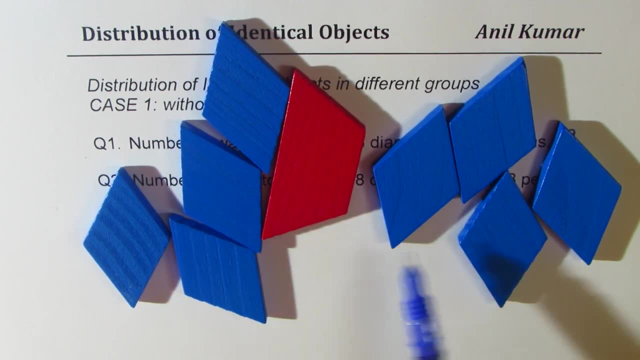 have now. what we have now is basically nine elements, right, eight and one we introduce now. the question is: we need to arrange all nine elements, out of which eight are same kind. so so what we know from what we have learned: nine elements will give us nine factorial 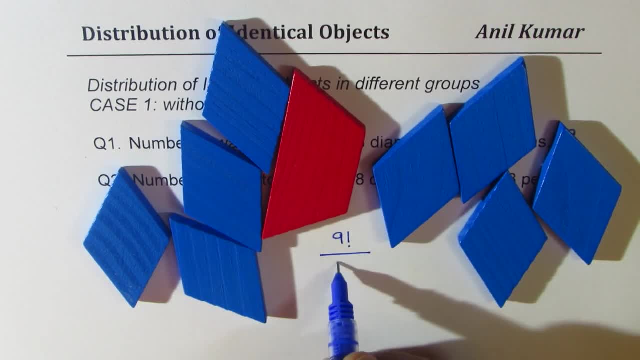 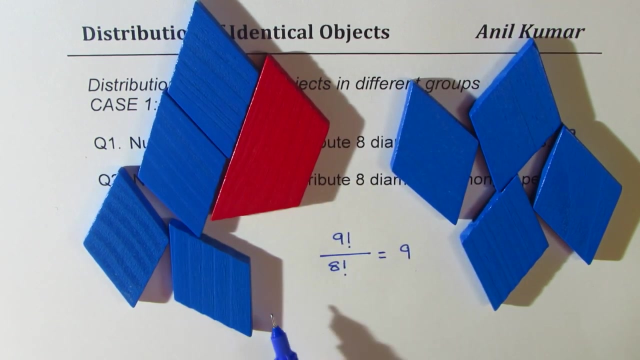 divided by eight of one kind means divided by eight factorial, and that gives you that, gives you nine right. that gives you what we wanted. do you see that? so? so we could get a result like this now in the form of combinations. we could also write this as: 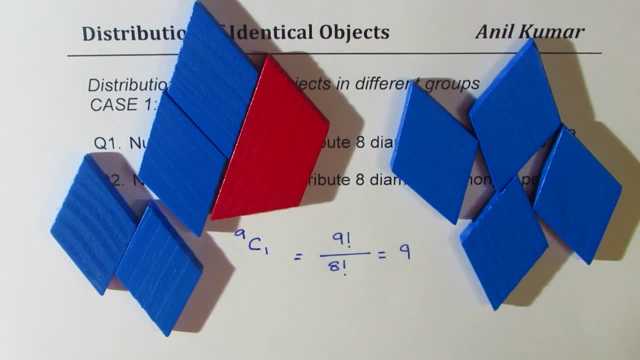 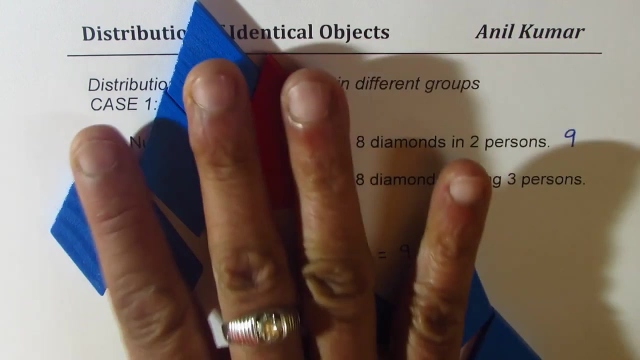 nine c one, correct, nine c one, and you can use calculator to calculate. you will get nine as your answer. now we're trying to, just, you know, get a formula some way or the other, and I think that works correct. now let's look into the second question, which is number of ways to distribute. 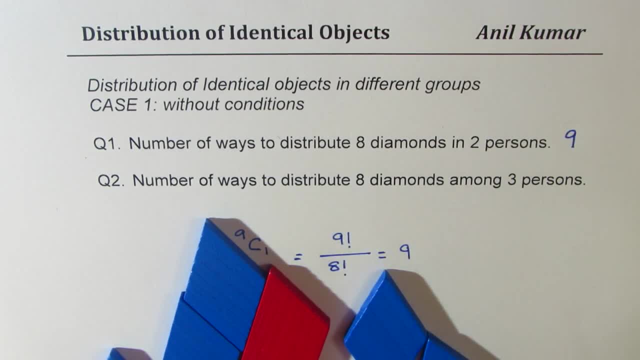 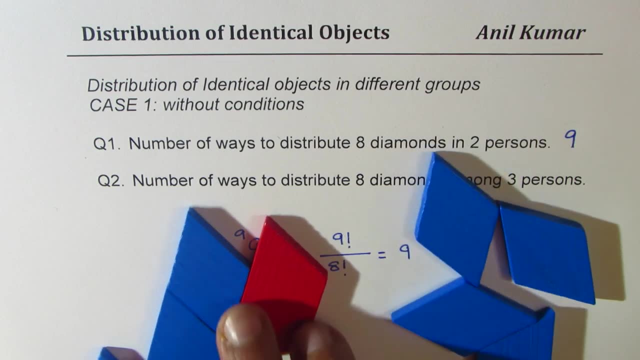 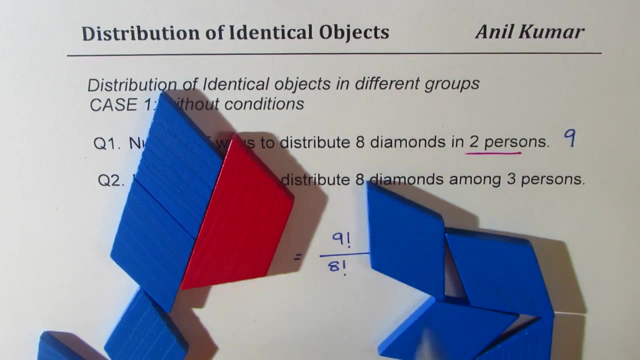 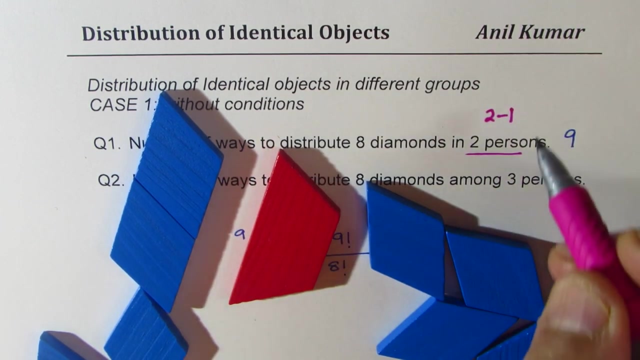 eight diamonds among three persons. now I have to distribute amongst three persons. well, let's try to understand this situation. in this situation we were interested in distributing among two persons, so P was two. we took two minus one as new block right? so so we introduced that and we had eight. 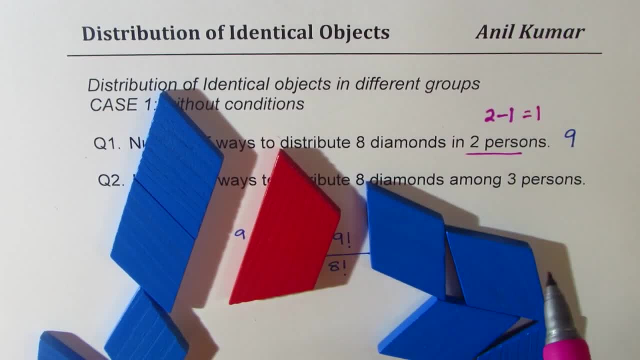 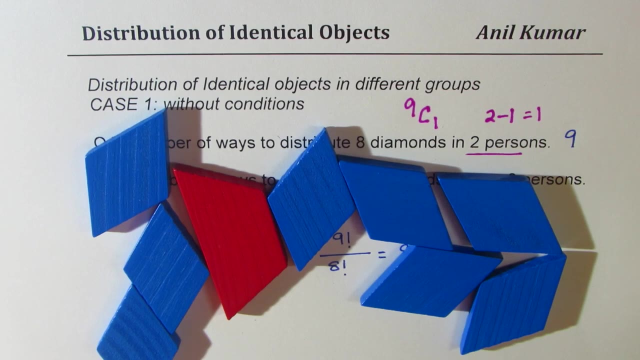 plus one and one is two. right now, given three is equal to seven plus one is equal to six, then let's assume that seven equals two plus one, right, so everything amongst three persons. now we can roasting them to be equal to seven plus one is nine. let't get it done. we put back the concept. it is still getting. 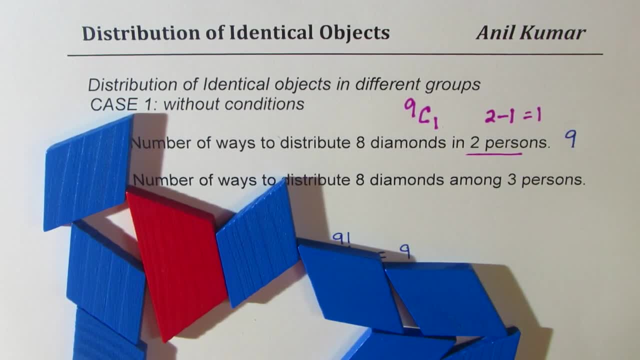 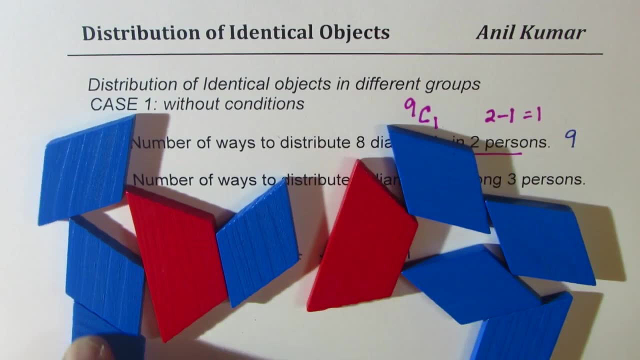 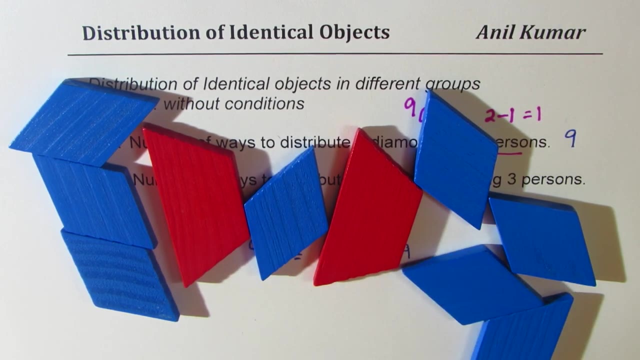 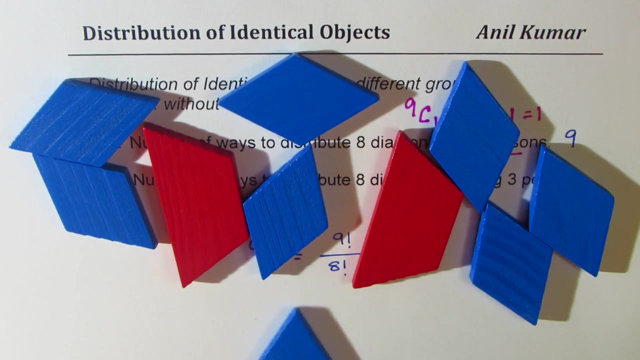 better for us success. so we have been interested in splitting the comes two columns and then it three ends. all three has seven ends shot instead of five. so how about this separator here? so I could make three different groups correct and accordingly I can actually make different number of combinations, as you can see right, just transferring one to the other place. 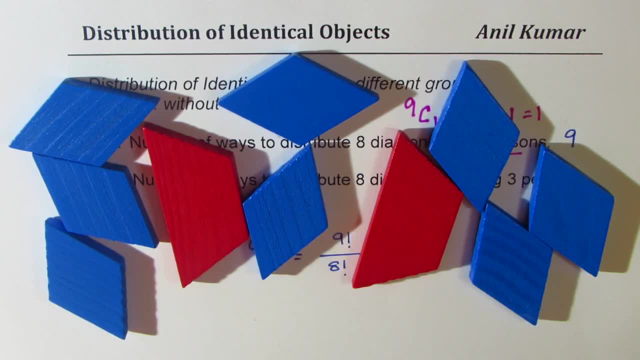 so that helps to visualize the situation. now, what do we have? we have in all eight plus two, which is 10. right, so we have 10 and we need to play around with these two. so 10 c2 becomes our solution, correct now? does it work for us? let's see, let's see. we could do like this. 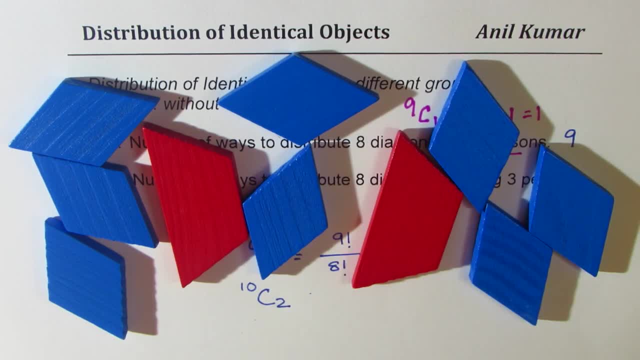 we have total 10 elements, right so we have total 10 elements, so we call them arrangement of 10. is 10 factorial, out of which these eight blues, eight diamonds, right so, and these two, two separators. so that is what we get. so, technically, we do get something which is 10 factorial over 8 factorial times 2 factorial. 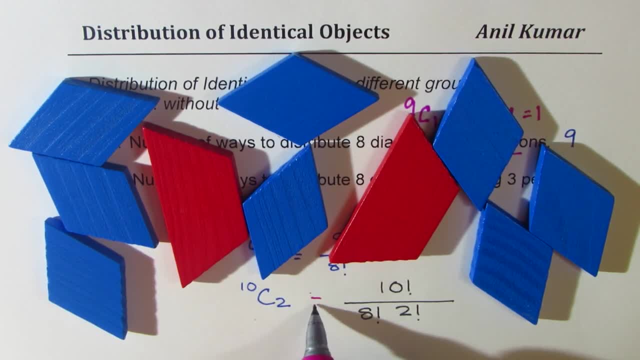 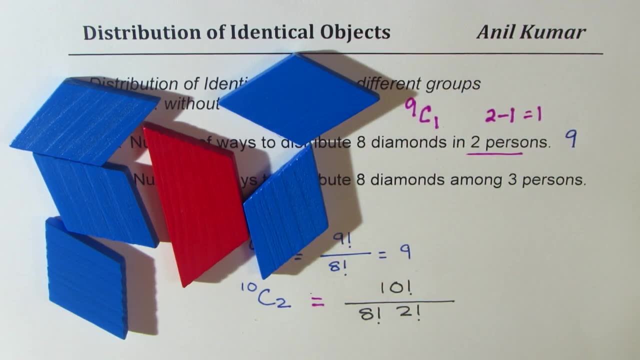 and that happens to be same as 10 c2. do you see that part correct? does it make sense to you? I think it does so. I think with this visual. I think it does so. I think with this visual. I think it does so. I think with this visual. 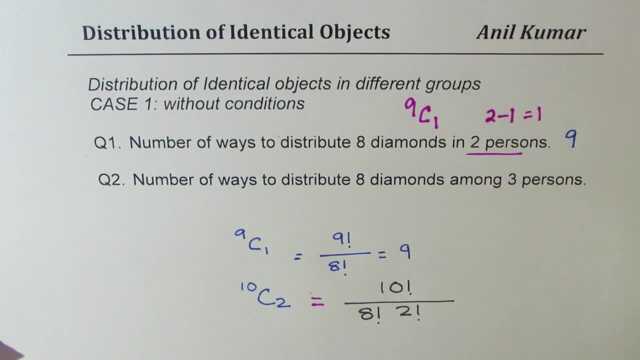 you could remember how we derived the formula right. so basically, if D is the diamonds, let's say: if D is the diamonds right and P is the persons, we are taking one less person right, so we are adding to our diamonds one less person right. so that gave us nine in the first case, ten in. 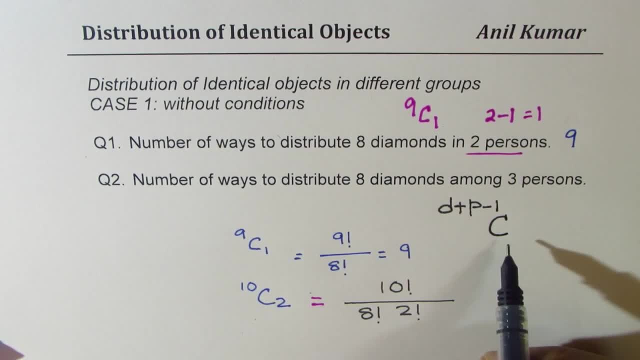 the second case. and here see how many intruders we had one less than the person right so. and here see how many intruders we had one less than the person right so we are getting a bigger refund of P minus 1. do you see that? so that becomes our formula for distributing identical objects when. 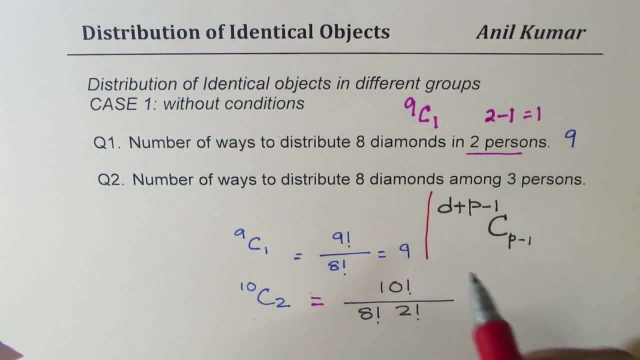 of P minus 1. do you see that? so that becomes our formula for distributing identical objects when there are no conditions. that is to say, we could give even 0 diamonds to a person, we could give one to any number. does it make sense to you, right? so this is a very important formula which we are derived, and I like 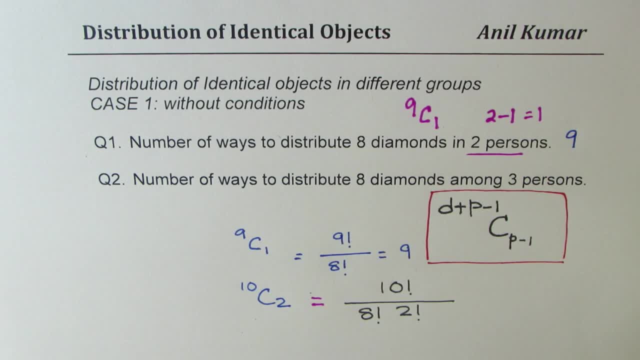 which we are derived, and I like you to go to this part once again so that you understand a little bit how toapper we have doesn't mean any numbers F, you know, and in that sense it is very simple to remember an example forward. it takes something there at what he has, to take two, несколько dice to determine exactly. 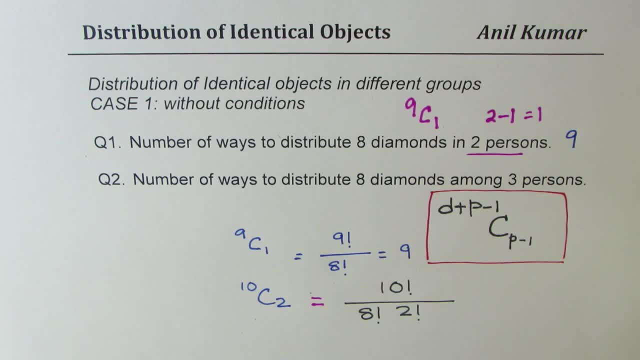 So that you understand this concept correct. And from here we are going to solve all the equations correct. From here we are going to solve all the equations. Now let's look into question number three, where we do have a condition. 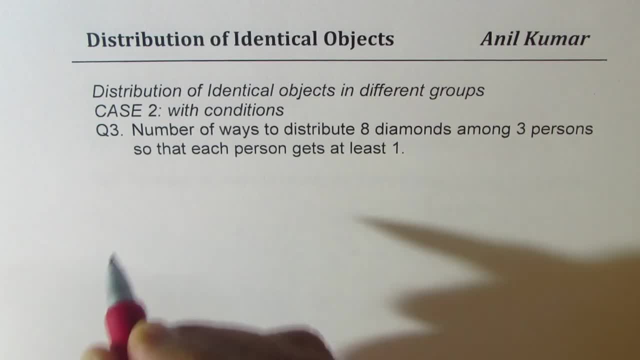 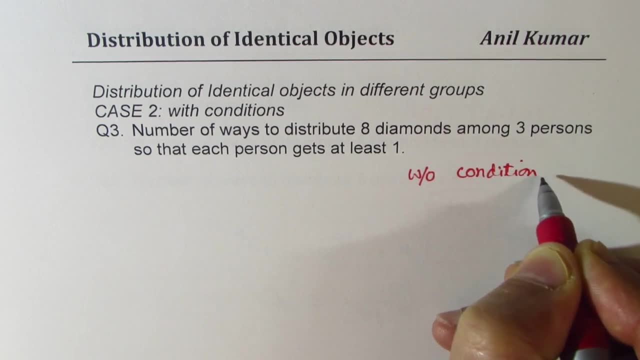 So the formula derived was- let me write here without condition- And the formula is: number of diamonds we are taking. we are adding p minus 1, c, p minus 1, correct? That is the formula which we just derived. 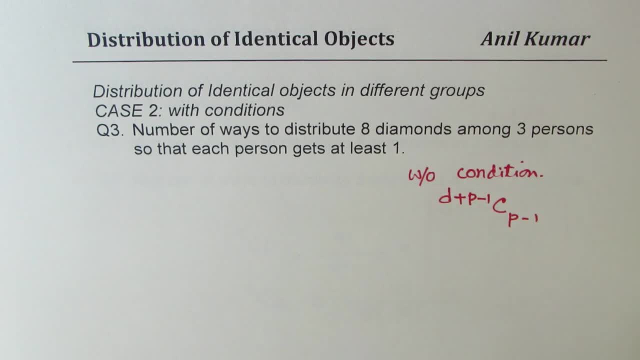 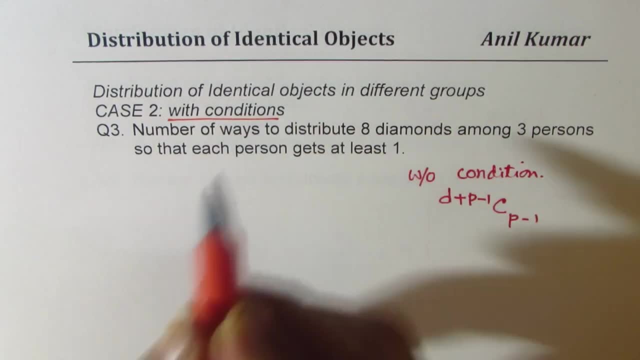 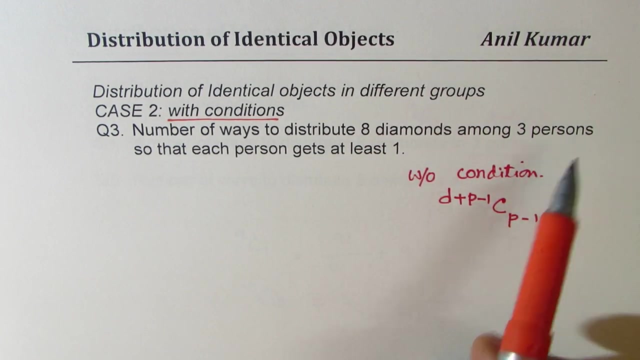 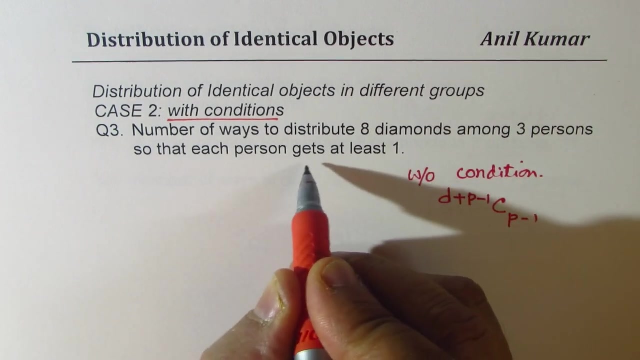 Now let us see how to modify this with given conditions, right? So question number three says case two with conditions: Number of ways to distribute two diamonds Among three people or three persons, so that each person gets at least one. Now we have a condition that they get at least one diamond each person. 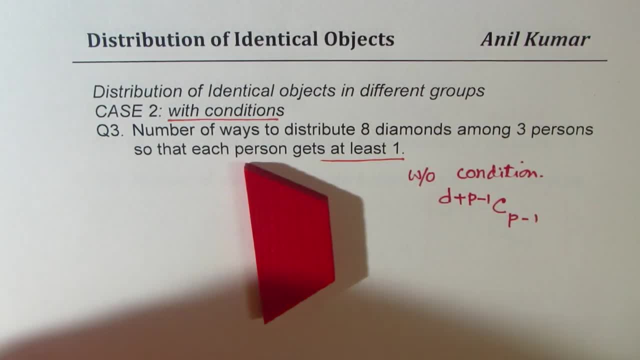 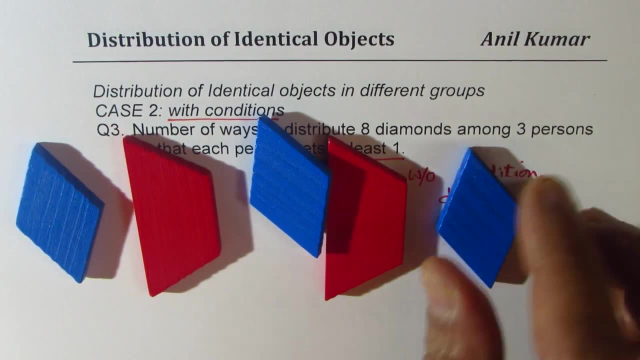 Well, so let's do one thing: We will again introduce our separators. correct, We introduce our separators. So these are the three groups. Let's give one to each, So the condition is met. Do you see that part? So what we did here was that. 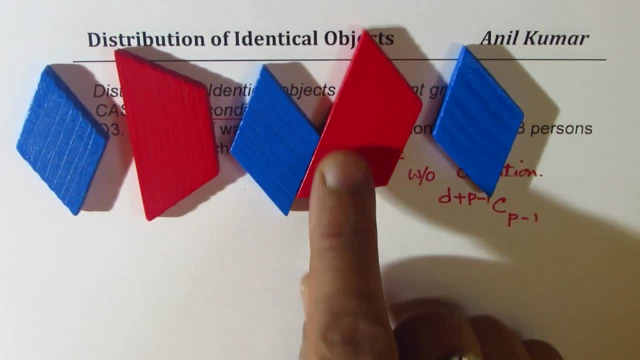 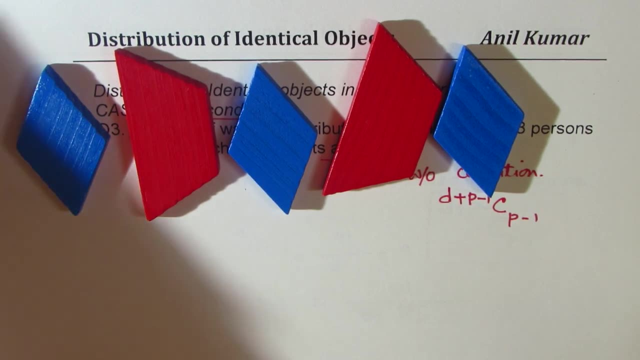 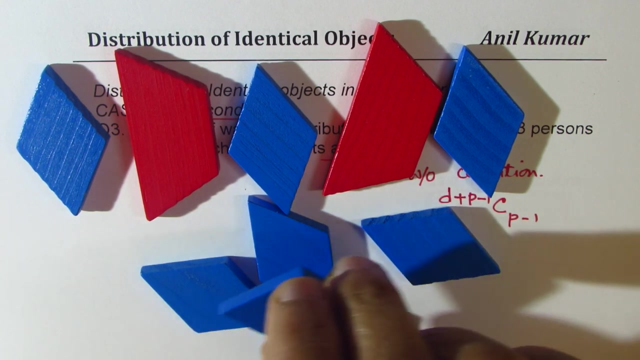 we have our separators and we just distributed one each, So the condition is met. All of them, all three- have got one each, correct? Now I could distribute these five any way I like, without any condition. 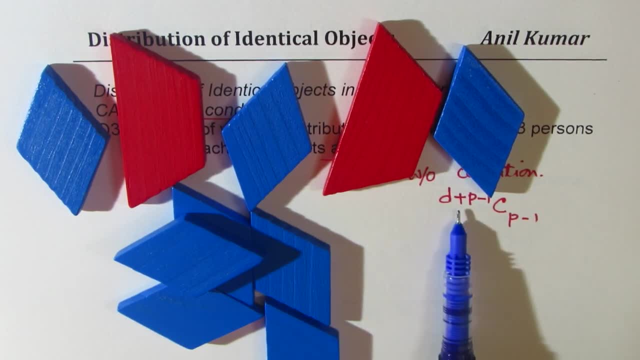 Do you see that? So that means, now I could apply this formula. The only thing is that I am left with only five diamonds, right? So the result is these five. number of persons: still three. So three minus one, which is these two. 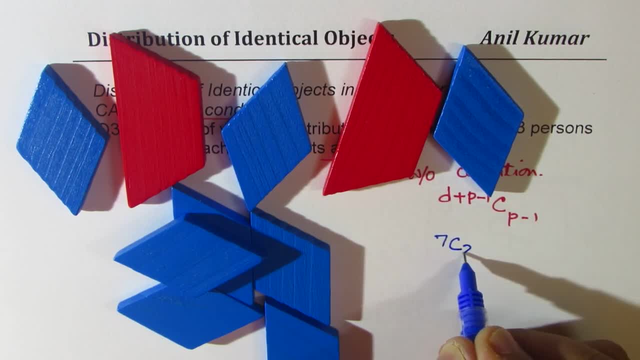 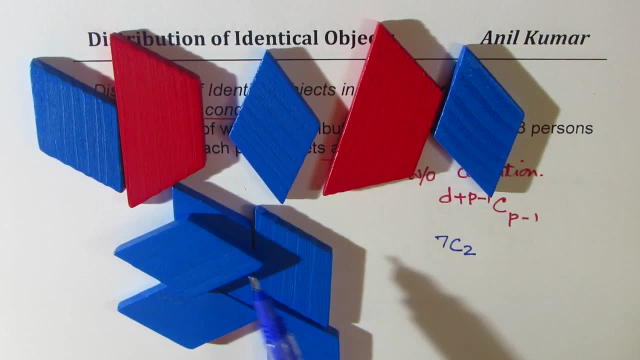 So we get seven. see two as our answer. Does it make sense, right? We already given one, So we have met the condition and we are left with five. Now this is without condition, right? So distributing five diamonds in three persons? 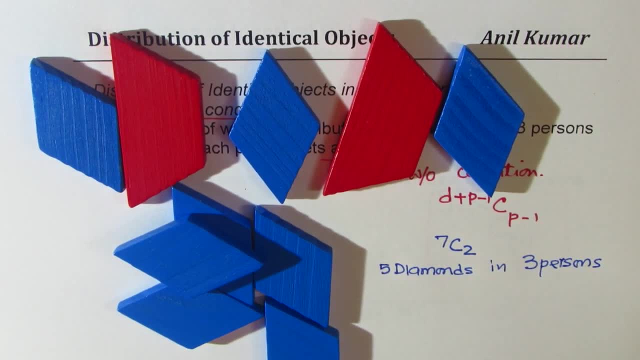 Correct. So that is seven, see two. So that is how we can actually apply our formula, which we just derived, to improvise the conditional cases also. Do you understand this part? So that's the beauty of it, correct? 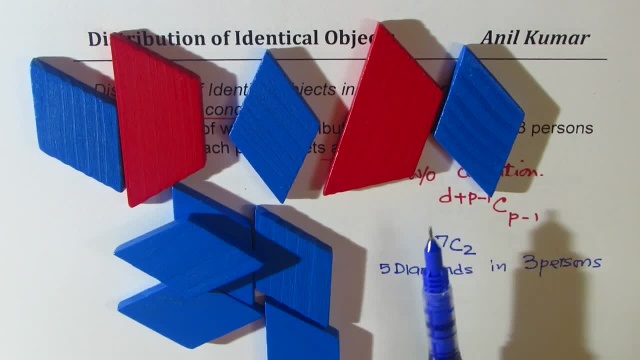 So we'll only work with one formula, which is number of diamonds plus number of persons, minus one, because minus one is the columns which divides right Into three different groups. In this case it should be two columns, correct? Now let's move forward. 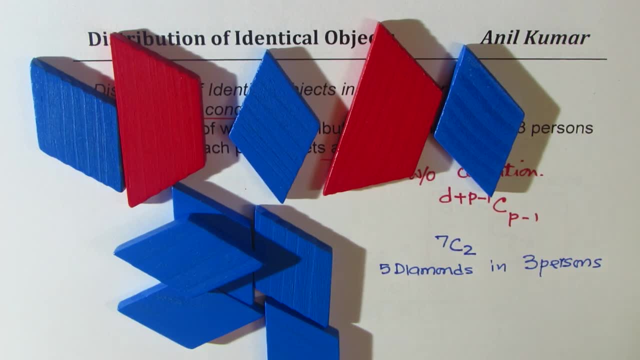 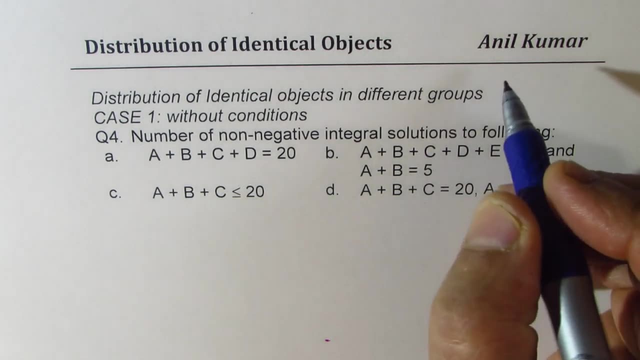 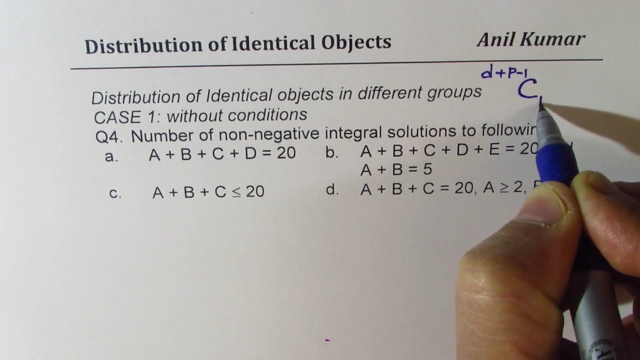 and then solve the equations from this particular logic. Correct Now, from our example on distributing diamonds to persons, we derived the formula, that is, number of diamonds plus one less person, combination is one less person. So those are the divisors, kind of. 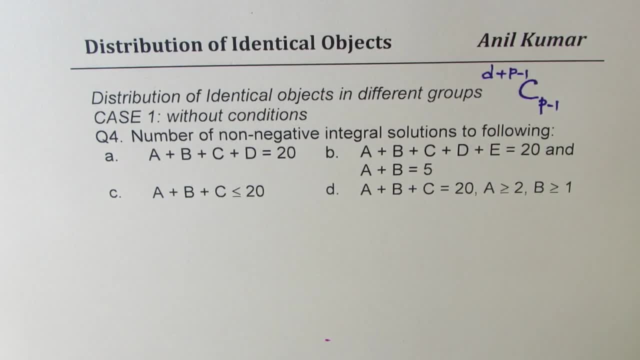 Is it okay. So that is the formula. Now let's see how to solve or improvise this formula for different kinds of equations. Now these are very critical questions. Question number four Determine the number of, so question number four is number of non-negative integral solutions to following. 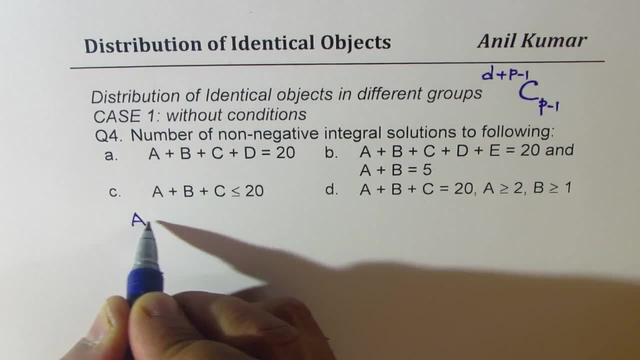 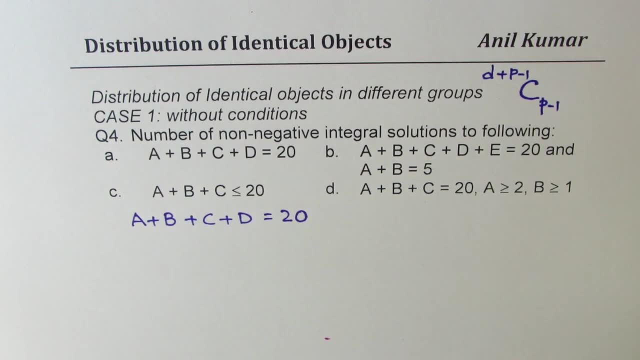 So we'll take the first equation, which is: A plus B plus C plus D equals to twins. Now, in this particular case, you can think like this: that we have 20 diamonds right, So we have something to distribute, right. 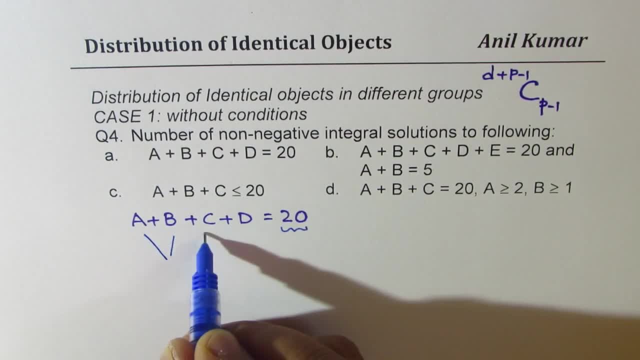 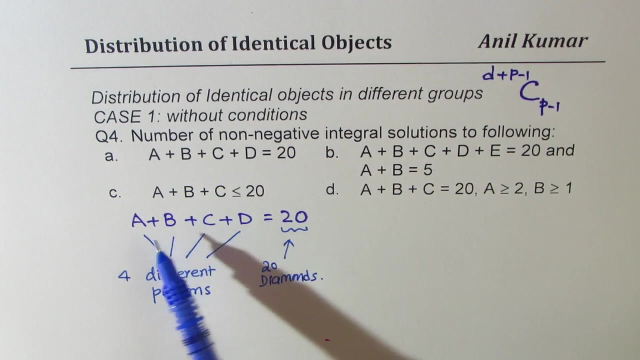 And these are four different persons, right? So these are. think like this: These are four different persons And these are 20 diamonds. Now, there is no condition. We could give all those 20 to one person. We could distribute them equally. 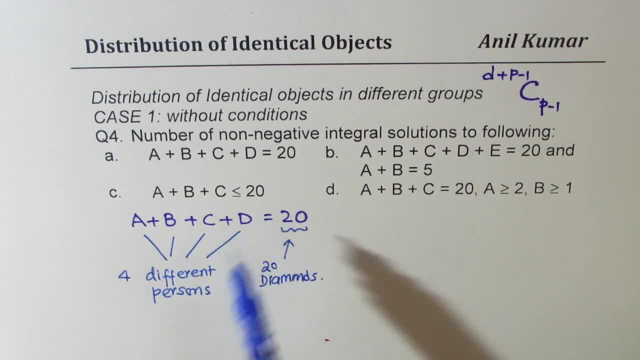 like five, five, five each or any way we like. Correct. Now, if I treat this like we treated our diamonds and persons, then what do we get here? Since there are four persons, I need three separators. correct, This time I need three separators. 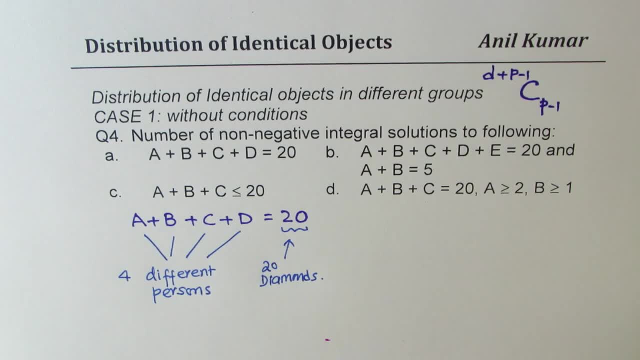 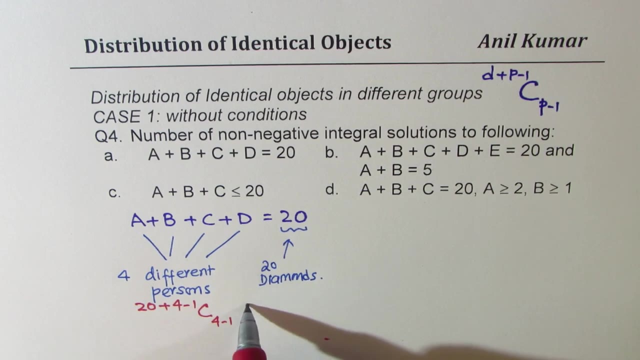 So. so the formula becomes: 20 is the number of diamonds, So we get 20 plus number of persons is four, four minus one C, and number of separators will be three, That is, four minus one, correct? So the solution will be 23C3. 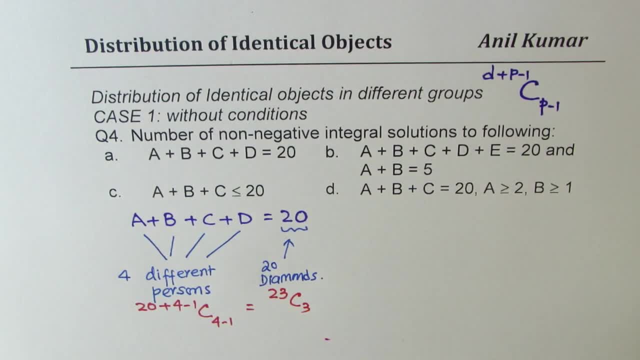 Does it make sense to you. So that is the trick: correct Immediately, you get the solution. Does it make sense Now? I hope the formula has been registered in your mind Right Now. here is next question. The next question is very critical. 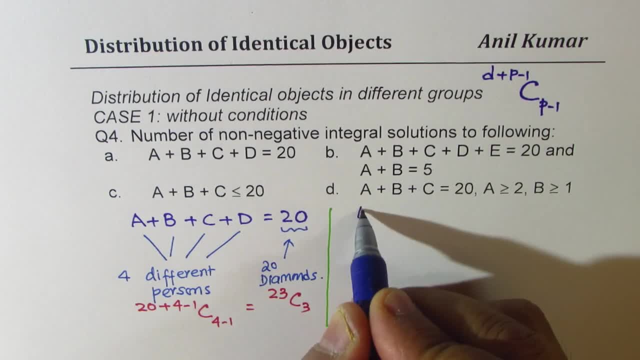 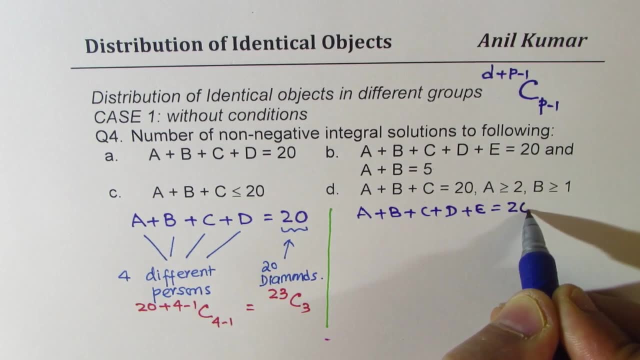 We have this time two conditions, that is, we want to say that A plus B, plus C plus D- okay, plus E- is equal to 20, and we have two conditions, and A plus B is equal to five. Now, both equations should be true. 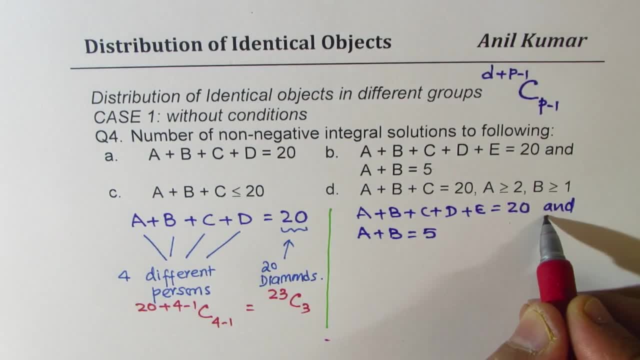 This is the AND condition which we have to work on: Correct. How do we solve such question? Think about it Now. what we can do here is that we can divide it into two parts, That is to say that let's treat it like this. 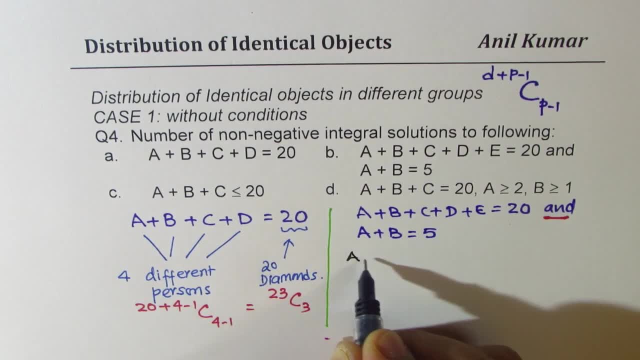 We want to distribute five diamonds among A and B and out of 20, what remains 15.. So C plus D plus E, they get 15 diamonds. You get an idea right. So two persons, five diamonds. so it is 5 plus 1, 6,. 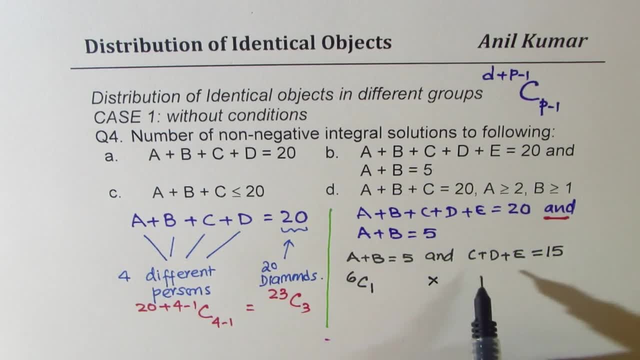 C1, AND means multiply, and this is 15 persons, 3, I mean 15 diamonds, 3 persons. that means two separators. so 15 plus 2 is 17, C2.. You get an idea. So the solution of second equation is: 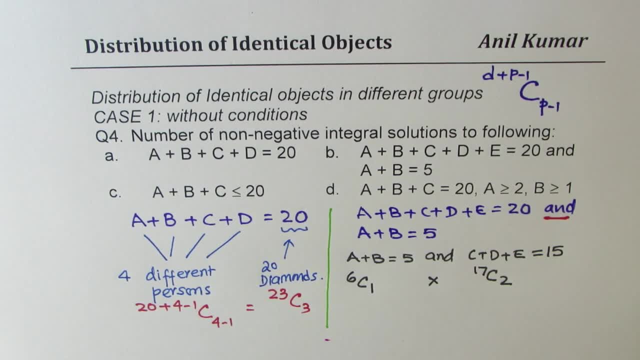 6C1 times 17C2.. Does it make sense to you? So that becomes the solution for the second equation, Correct? So I hope you are kind of appreciating it right. So it is that good. Now we will do part C and D. 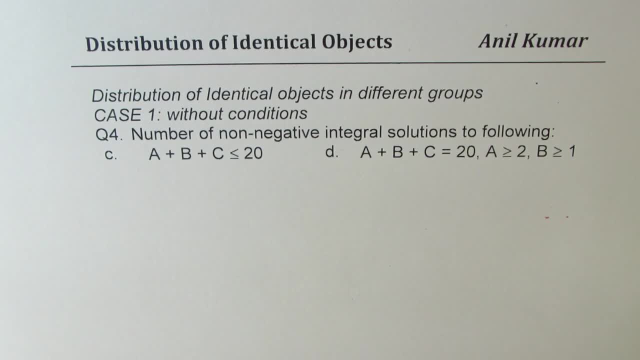 which are very tricky equations, And let's see what additional things we have to improvise to use this beautiful formula of distributing diamonds to persons, right? So the formula is: diamonds plus persons minus 1, C persons minus 1.. Okay, that's the formula. 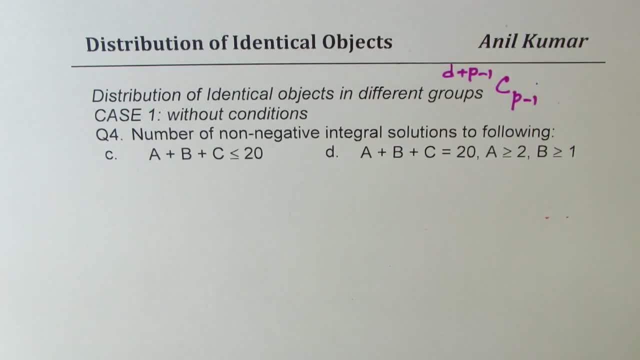 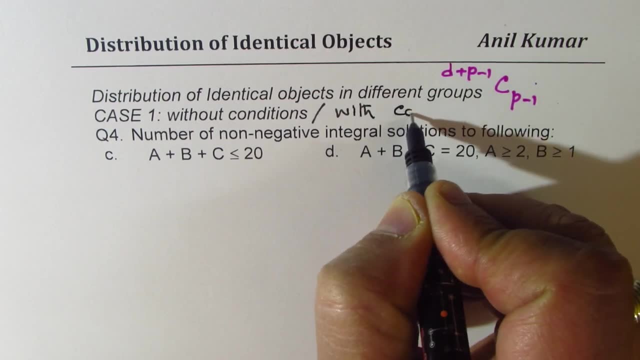 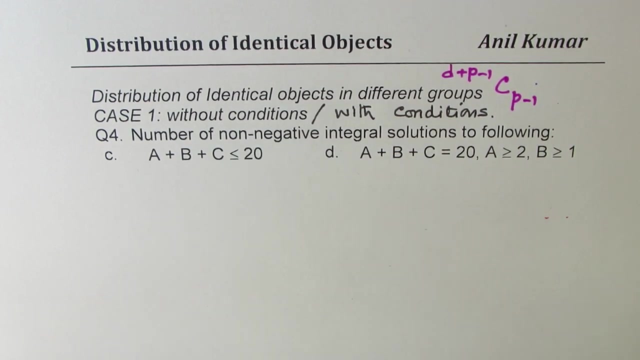 Okay, Now it is combination of case 1 and 2. So we are doing without condition and we are also doing with conditions. See E plus B plus C is less than equal to 20.. Now it is not equation, It is now an inequality. 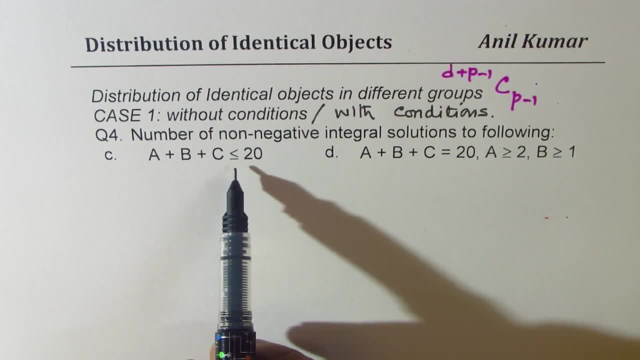 How do we solve this Now? to solve this, it really means less than equal to 20, means it could be 0, it could be 1,, 2,, 3,, 4, like this correct Now to convert it into an equation: 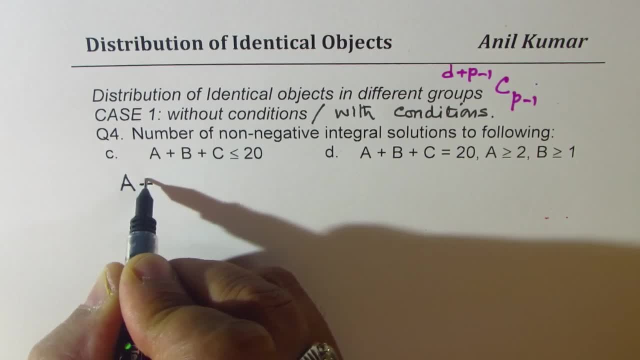 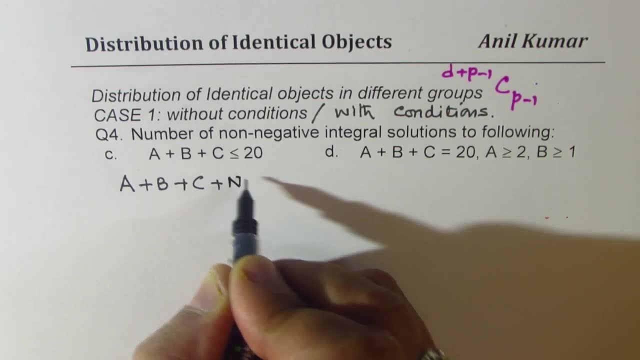 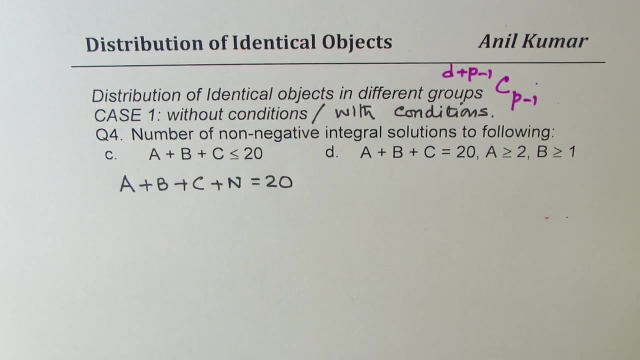 see the change which I am going to do. I am going to treat this as A plus B plus C plus. let me use another number here. let's say N is equal to 20.. So we can add some number so that it becomes 20 all the time. 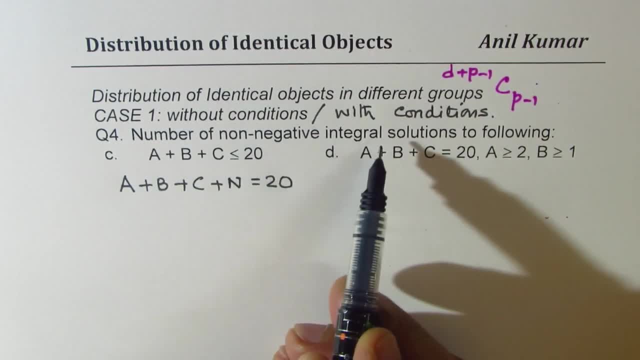 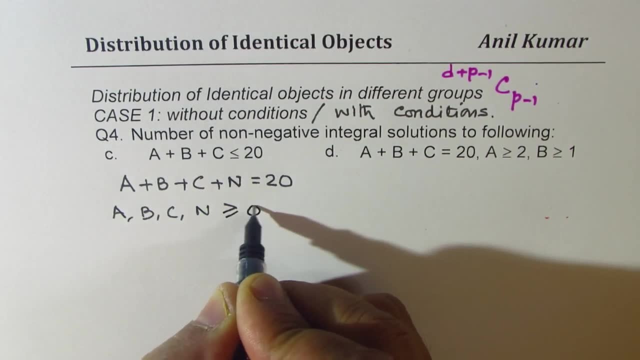 Do you see that Now, in this equation, when we say non-negative integral solutions, we know A, B, C and N, all should be greater than equal to 0, right, Non-negative. So basically, if you look into it, 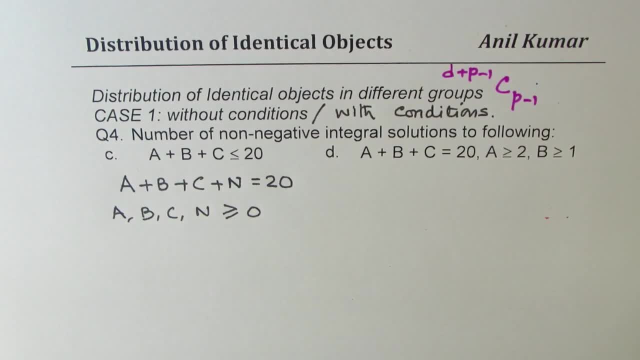 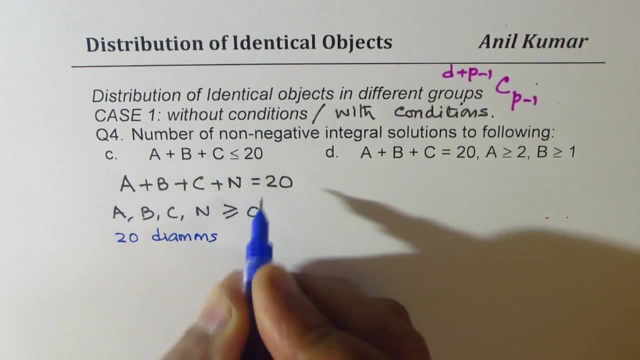 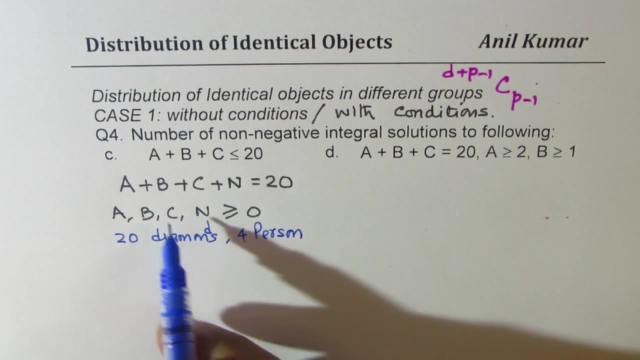 we again have 20 diamonds right. Think like this: What do we have? now We have 20 diamonds and this time we have 4%. So if I have to distribute, I need 3 separators, right- 3 separators. 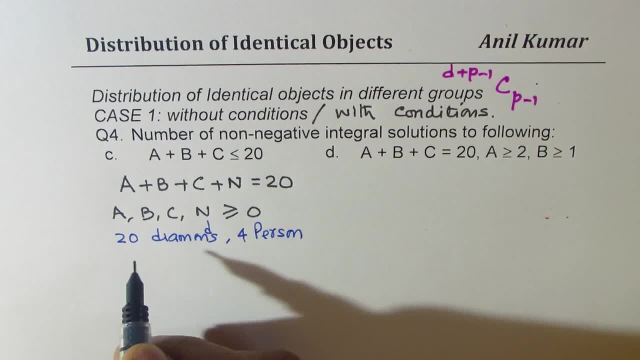 So I have to add 3 to this. So what do I get If I add 3 to this? I get 23 C and there are 3 separators. That's the result which you get, the same by applying the formula. Does it make sense to you? 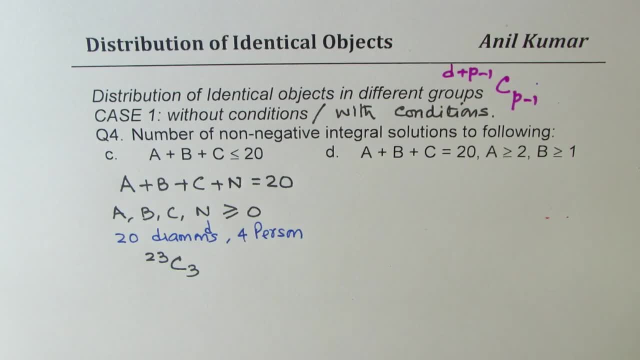 Now that's the tricky part, correct? This is how we could improvise our learning into different conditions, and that takes you to a much higher level. We'll actually take more critical equations and different examples, which you could see in IIT-J papers. 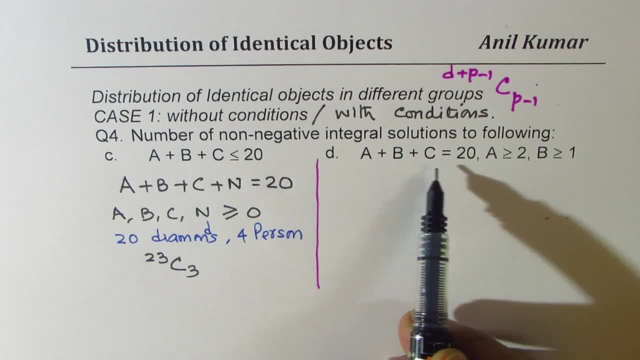 Now let's look into the last question. A plus B plus C equals to 20, but we are giving a condition that A should be greater than equal to 2 and B should be greater than equal to 1.. That means C is greater than equal to 0,. 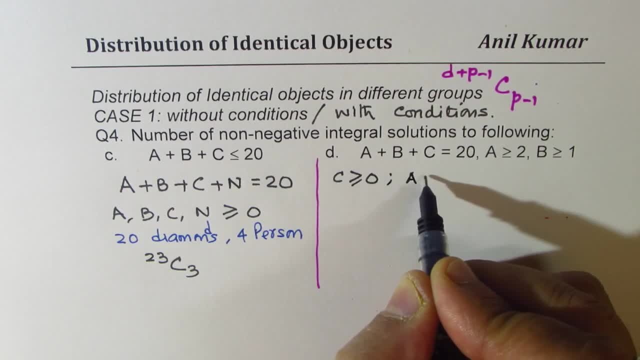 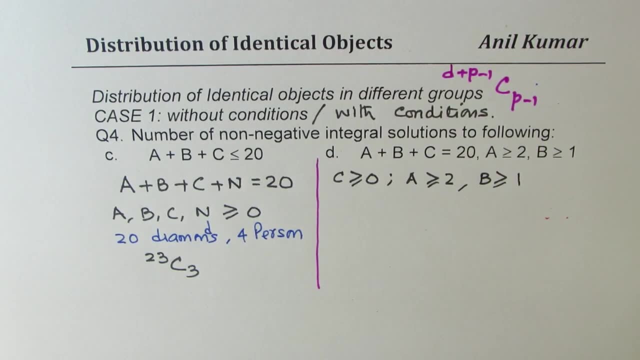 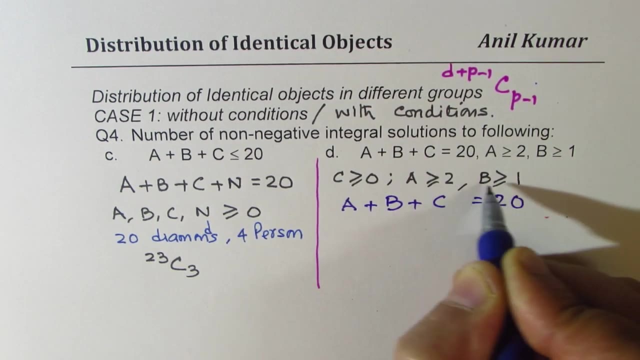 no condition, basically, and we are saying A is greater than equal to 2 and B is greater than equal to 1.. Okay, So the question here is that A plus B plus C should be equal to 20 with the given conditions. What should I do? 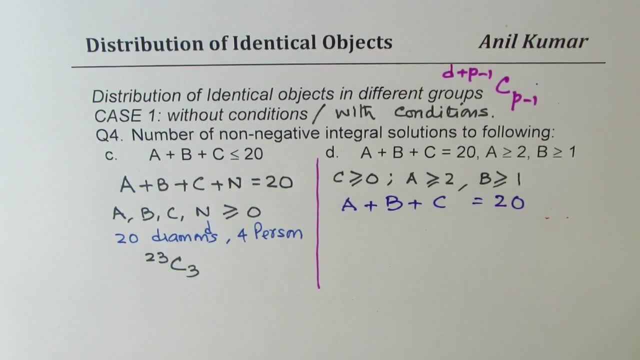 So, as we did in the very first example with condition, we'll actually give two points to A, that is, two diamonds to A already one diamond to B, So we have already given 2 and 1.. So we're left with what? 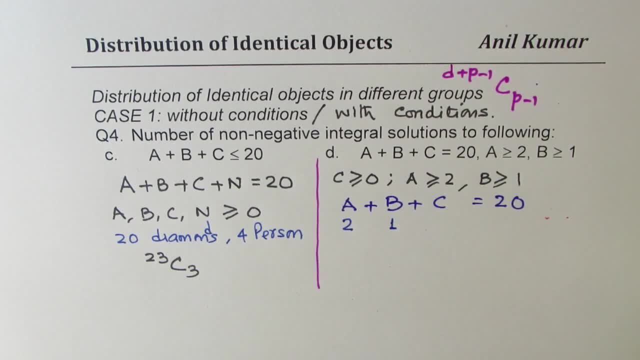 We're left with 20 minus 3.. So we get a new equation, which is A plus B plus C equals to 20 minus 3,, which is 17,. correct: A has already got 2, right: A already has got 2.. 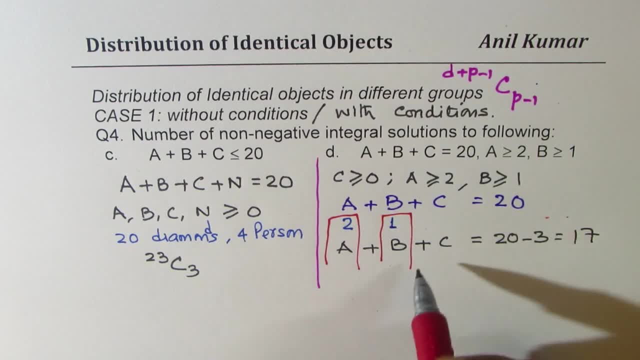 So that's it. B has got 1.. So that means we have met the condition. Now we have 17 diamonds to be distributed in three different people, So two separators. so that means 17 plus 2 is 19 C2.. 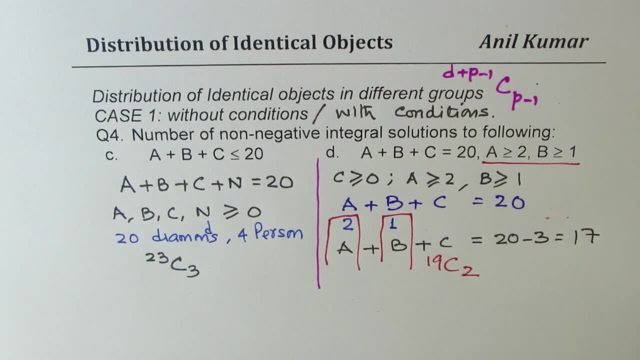 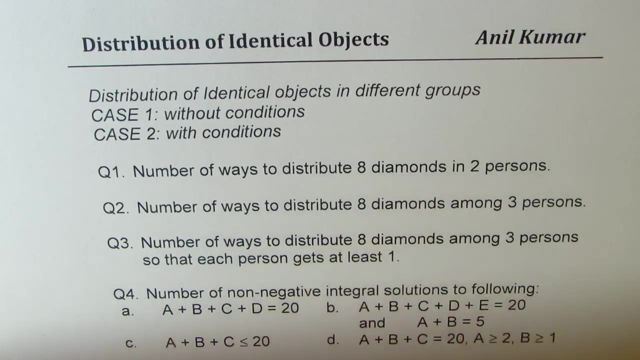 That becomes the solution for the given question. Now does that make sense to you, right? So we actually solved all these questions in no time. Now let's look into our questions and write down the answers. I would actually like you to pause the video. 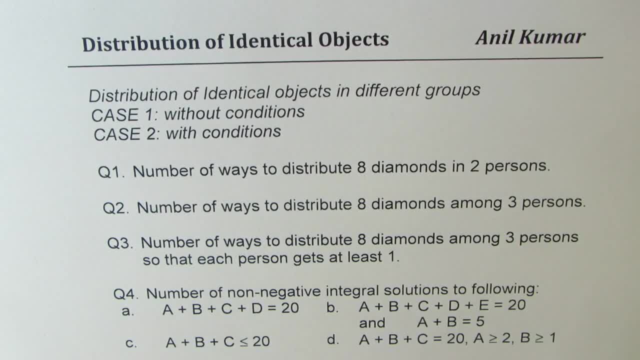 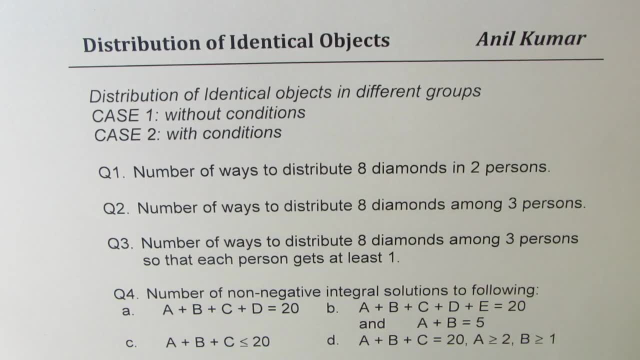 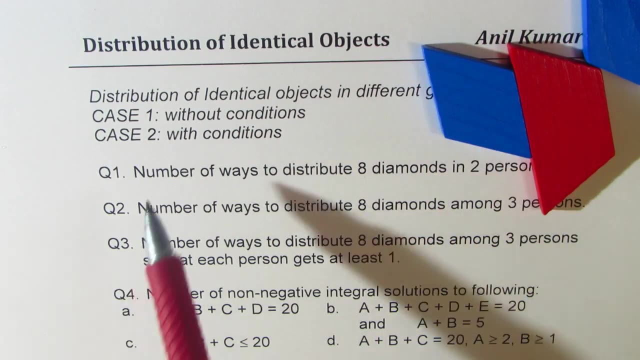 and answer all these questions now. okay, Take a minute, Let's go through them once again. So we talked about identical objects, which were diamonds- for us, right, These diamonds. And then we had these separators to separate them With and without condition. 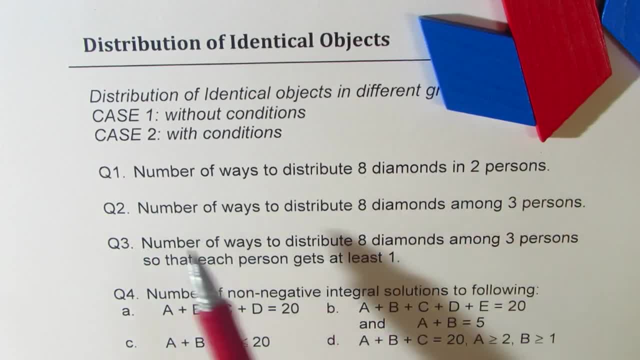 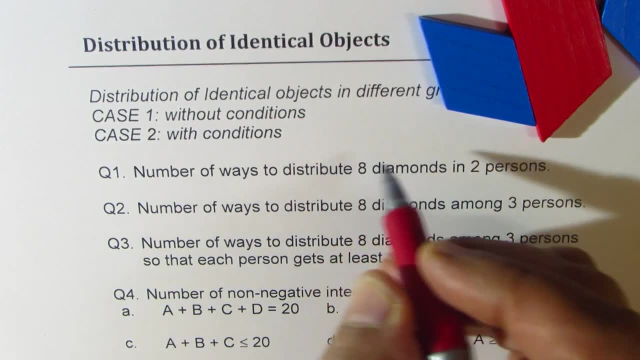 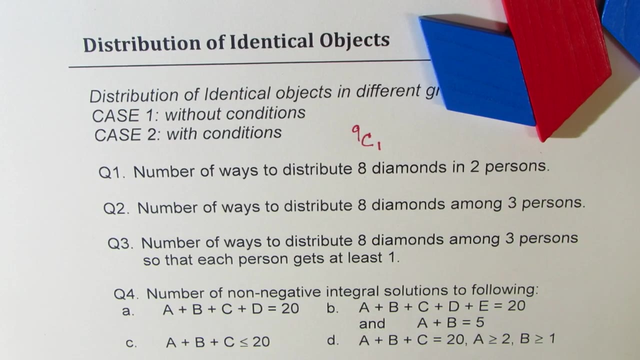 First two examples are without condition: Number of ways to distribute 8 diamonds in 2 persons. So we need 1 separator, So we get this time 9 C1.. There were 9 ways, correct, The second one. The second one is: 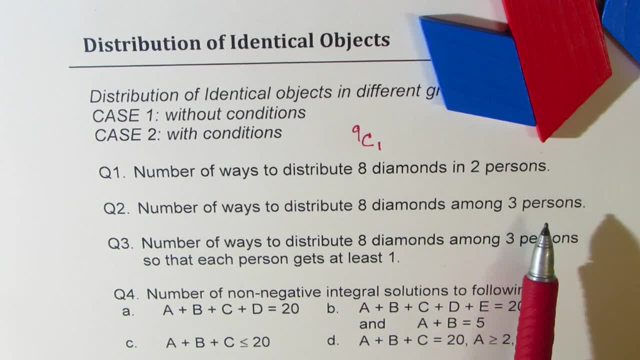 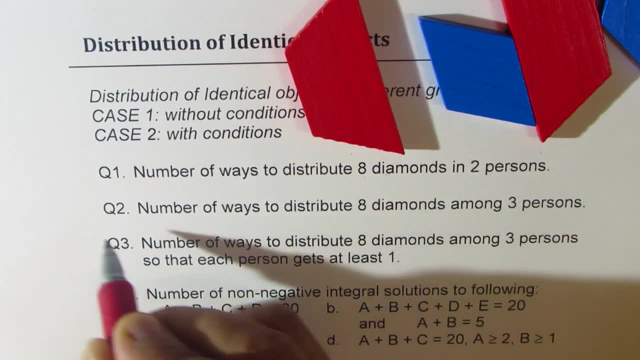 number of ways to distribute 8 amongst 3 persons. So for 3 persons we need 2 separators, right? So we added 2 to 8. So we got 10 for this, right? So we got 10 for this. 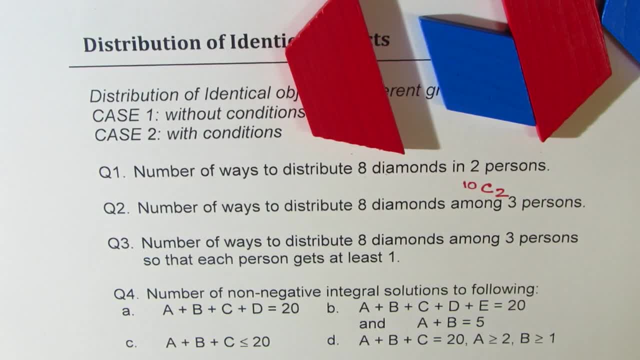 Let me write here 10 C2.. That was our solution, correct. Now in the third case: number of ways to distribute 8 diamonds amongst 3 persons so that each person gets 1.. So we gave 1 to each. 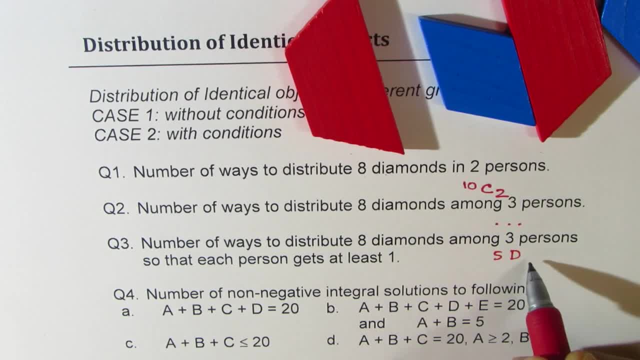 So that means we are left with 5 diamonds. So it is 5 diamonds and 3 persons right, So 2 separators. So we get 5 plus 2 is 7. C2. Does it make sense to you, right? 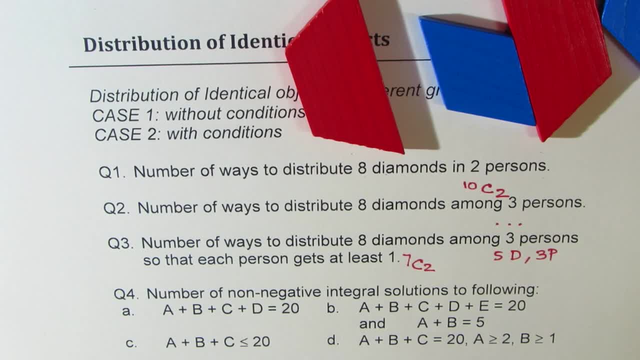 So we got 7 C2.. The answer for question number 3.. Now question number 4 is to solve an equation where the sum could be 20.. Any numbers could be distributed Non-negative. So we are saying in this case, A, B, C, D are all non-negative. 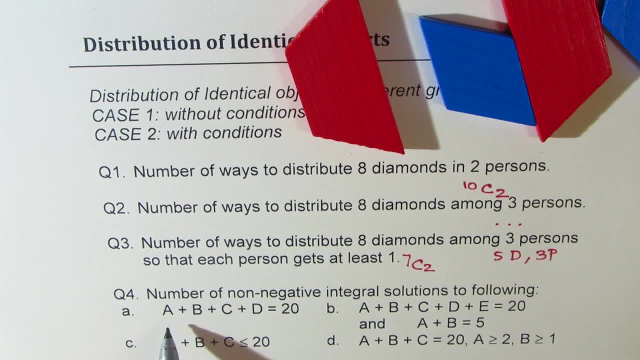 Means greater than or equal to 0. Okay, They could be 0 also. Now think about 20 diamonds, 3 separators. So we get here. in this case, we get 23 C and 3 separators. Got it correct. 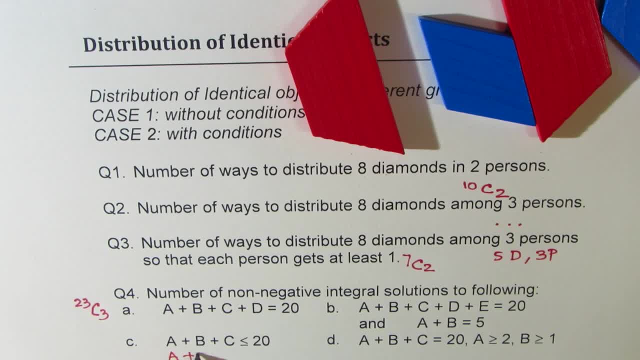 In this case we introduced another. So we wrote this as: A plus B plus C plus D equals to 20.. Correct, So we got 4.. So we need again. so it becomes kind of same right. So we again get 23 C3 as our answer. 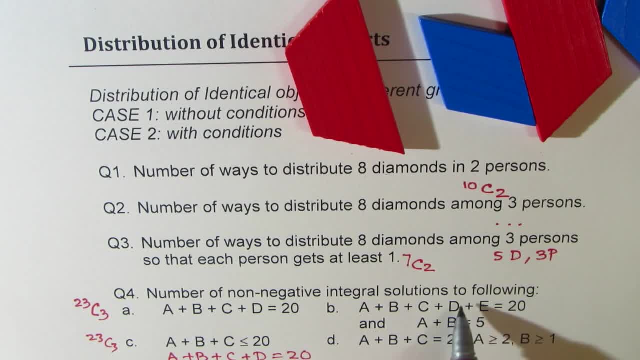 Okay, great. Now in this particular case, we have 2 different conditions. So we are working with 2 people getting 5 diamonds and 3 people getting 15.. So 2 people getting 5 diamonds. 5 diamonds and 1 separator means 6.. 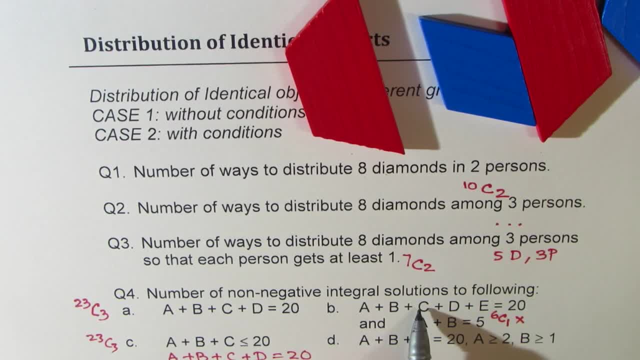 C1 times Here 3,. these 3 will get 15, right. So 3 means 2 separators, 17 C2.. Just multiply, get your answer. The last one, A should be 2, B should be 1.. 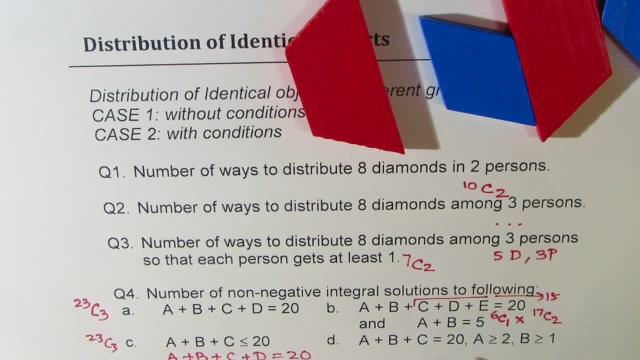 Let's give 2 to A, 1 diamond to B, We are left with what? 17,. right? So balance 17 amongst 3 people. So that means 2 separators. So we get 17 plus 2 as 19 C2.. 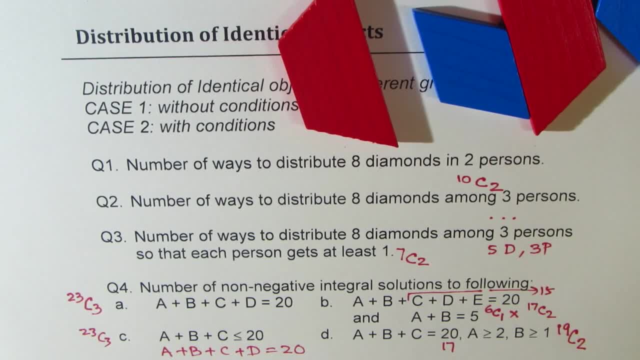 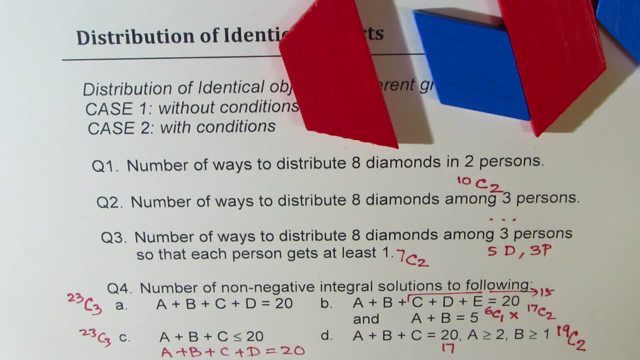 That's the answer, So I hope that makes sense right? So that is how you could do the cases which involve distribution of identical objects with or without conditions Does make sense to you. Feel free to write your comments and share your views. 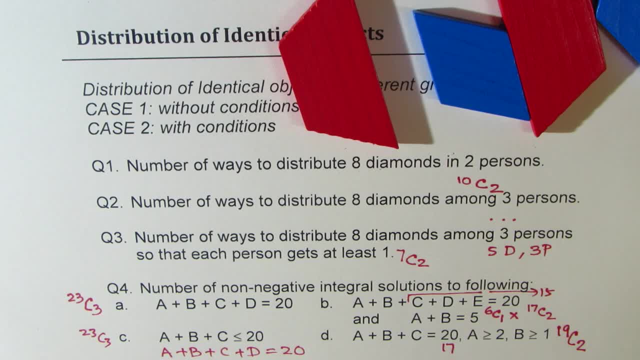 We will take up more videos on these tricks and I hope they really help you. Thanks for watching and all the best.